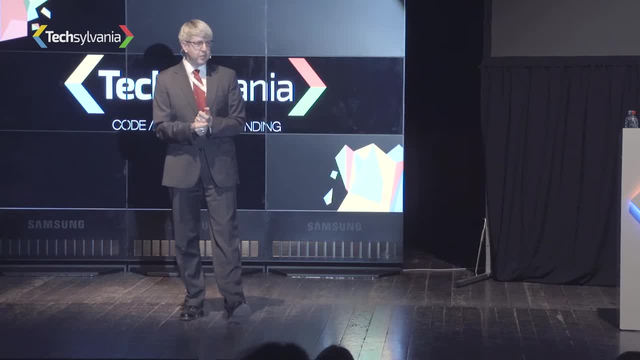 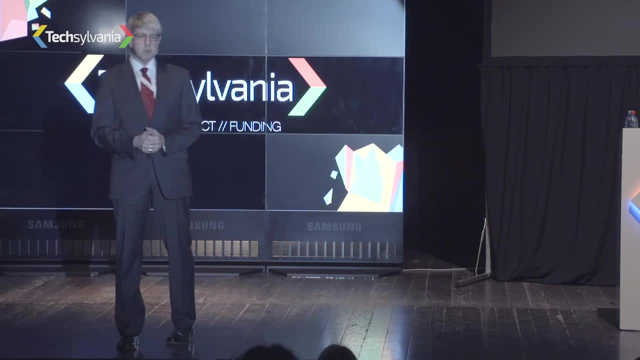 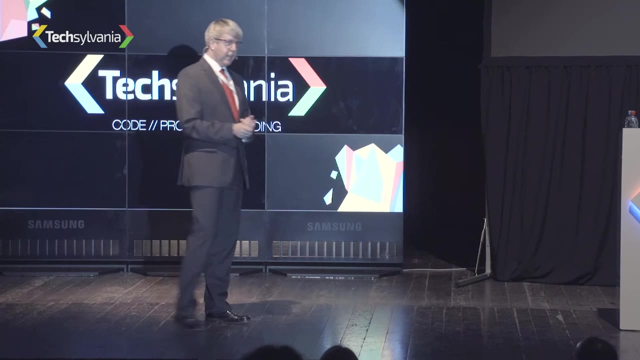 An idea. It's also laden with a lot of negative thoughts, And you have heard Stephen Hawking talking about that. we will lose two AIs at some point. Well, it's a bit time until then, And we always discussed what we do with our tools. 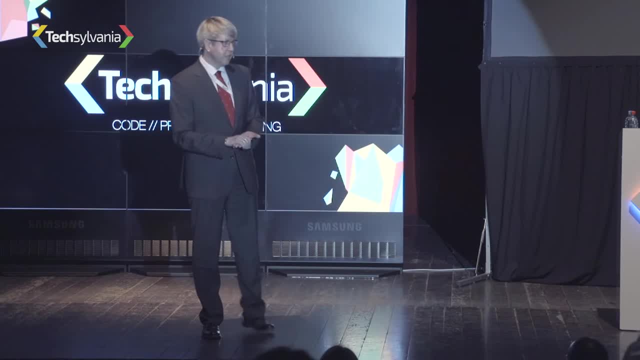 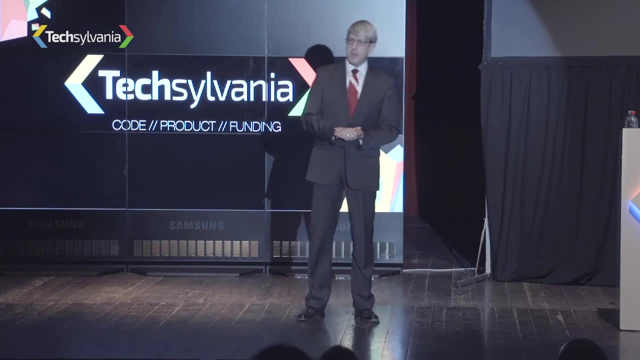 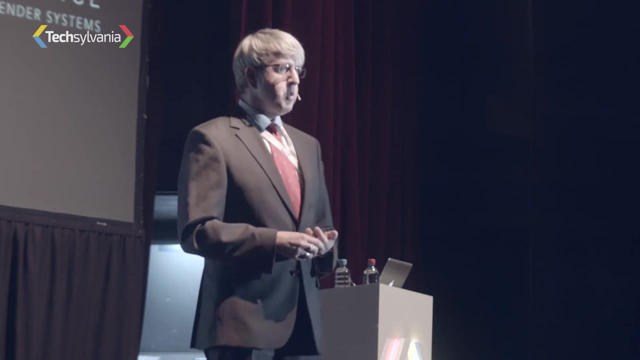 You know as well as I what you can do with a knife. You can use it as a tool, you can use it as a weapon. Same for AI, And there are lots of problematic decisions out there. We, as a public as well, have to think about what we want to do there. 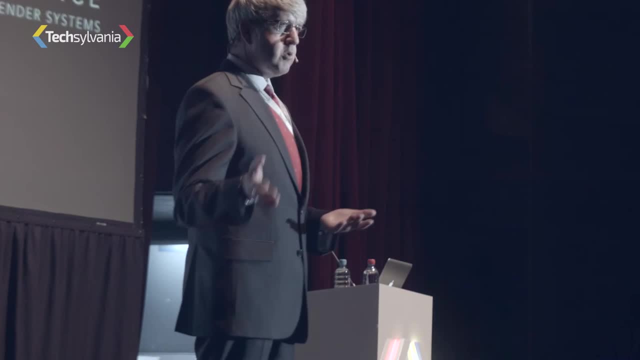 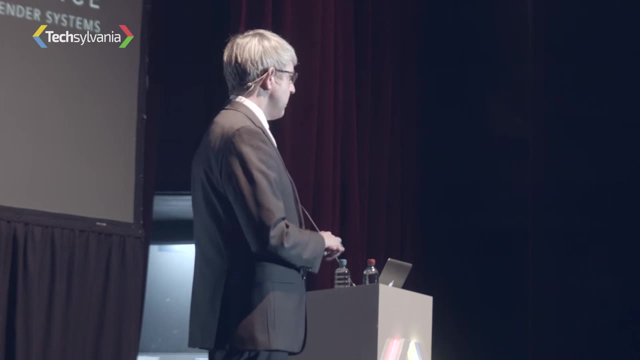 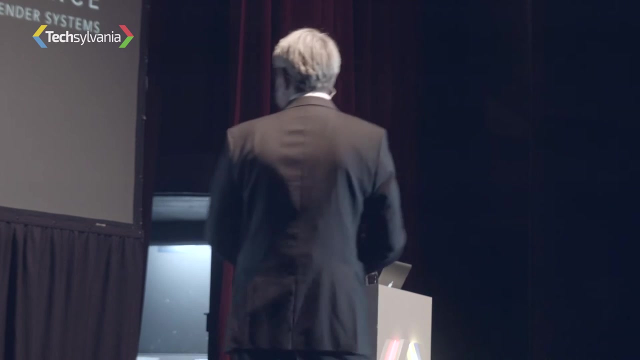 Looking at the NSA, GCHQ, Looking at drones being not only remote controlled but being able to decide autonomously. Do we want to have that? But I'm technology, I'm a technology optimist, So I want to introduce you to case based reasoning. 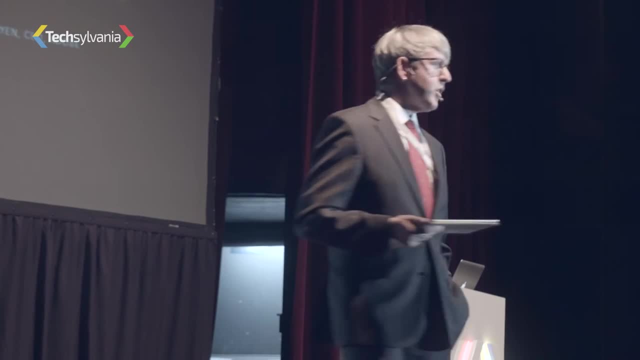 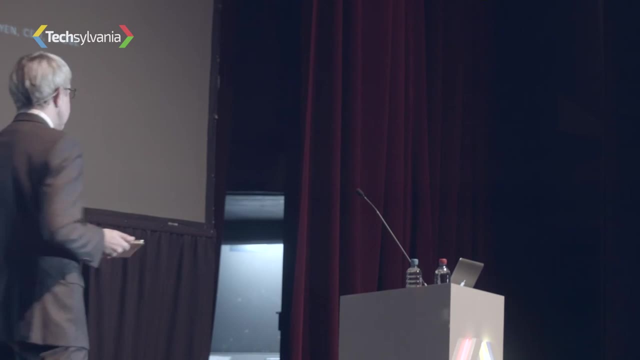 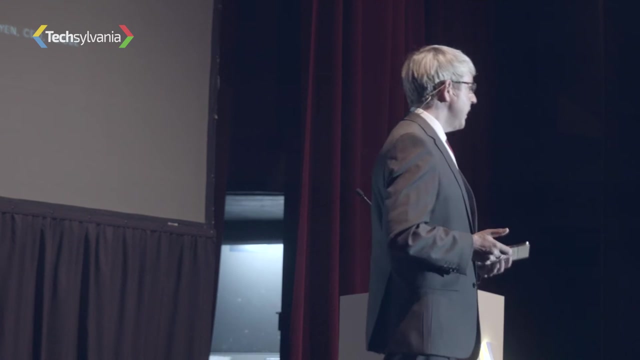 Listening to the Adobe keynote last year struck really a chord with me. So we as consumers expect relevant, interactive, personalized material, wherever we are, By the CEO of Adobe, Shantanu Narayan. That's what AI is really good at: It's helping you. 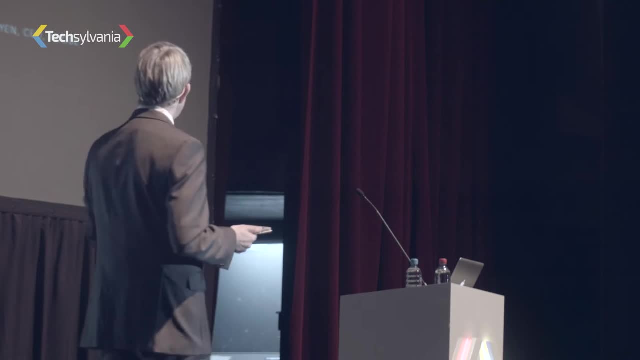 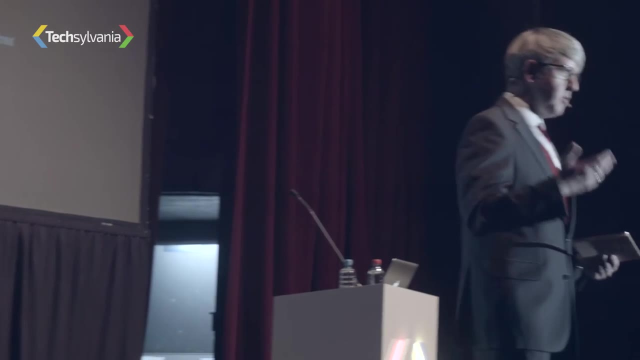 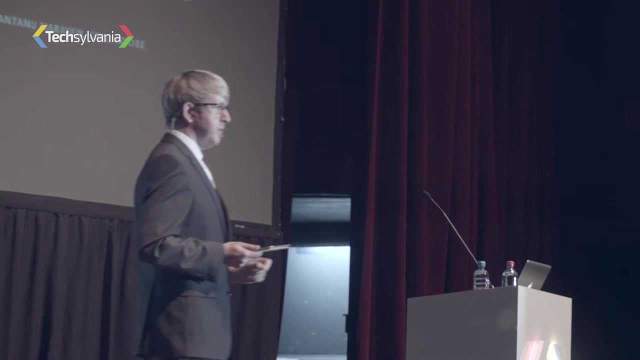 With this interactive bits, the personalized material, gaming and all these kind of methods that you bring in into your application to make the customer experience more enjoyable, And where case based reasoning is especially good is helping with the relevant bit To decide something relevant, something similar to what you need. 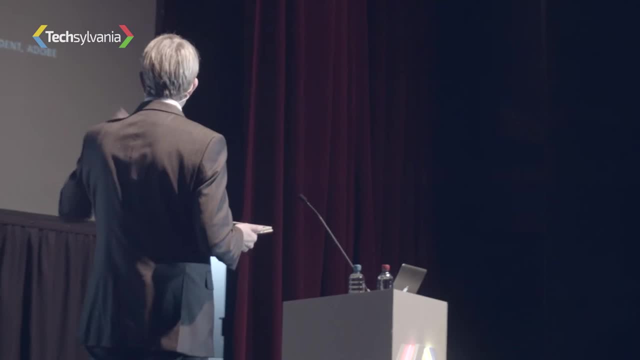 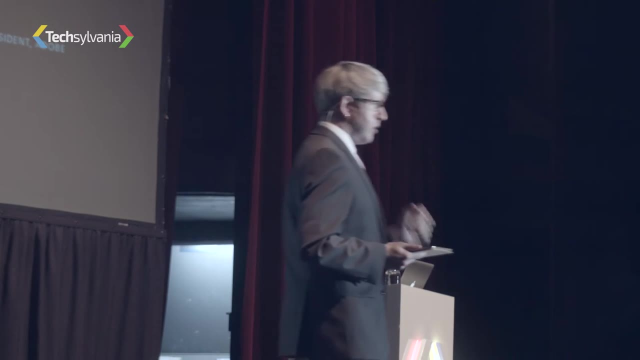 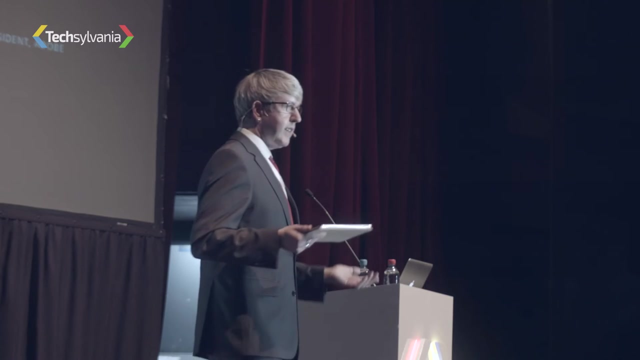 And the CEO was backed up by David Vardwani, the senior vice president of Adobe. The new frontier is experience. It's about cross selling. It's about cross media marketing, branding, shorter cycles being available to deliver that in shorter time. 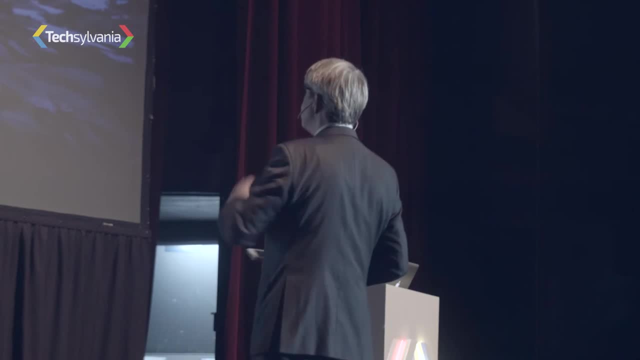 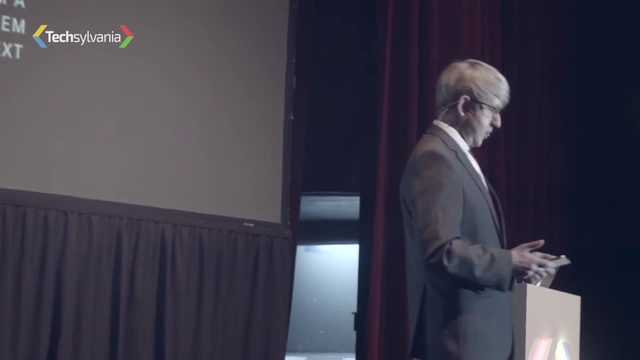 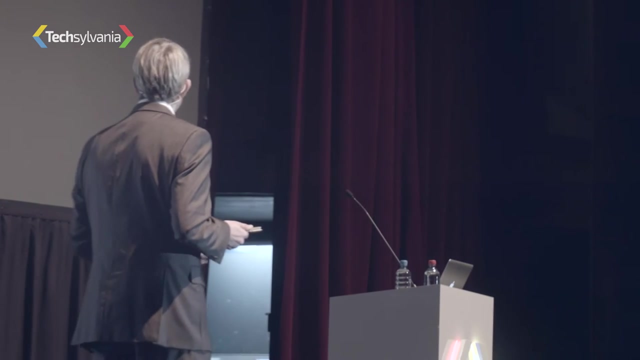 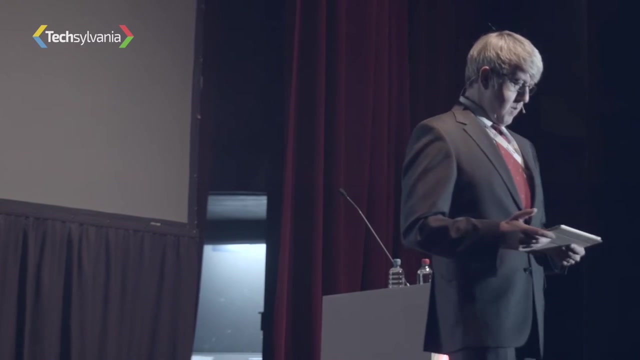 But what they all talk about is this kind of experience, right Like an unforgettable trip somewhere. That's not what I mean. It's about specific knowledge obtained from a specific problem solving context. That is really valuable, usable knowledge. That's something we can harness. 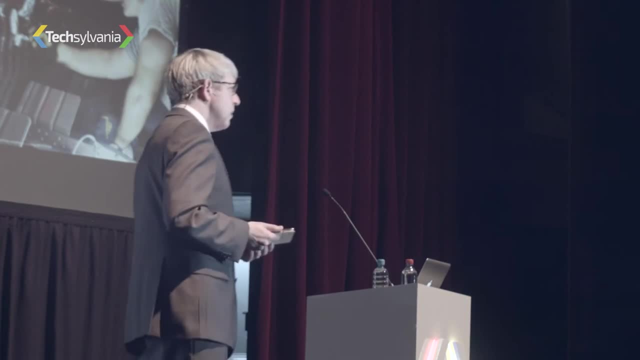 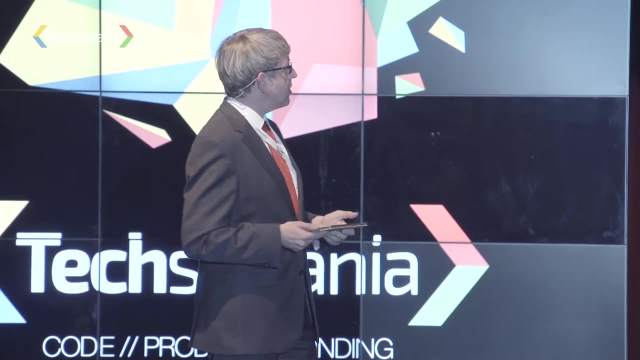 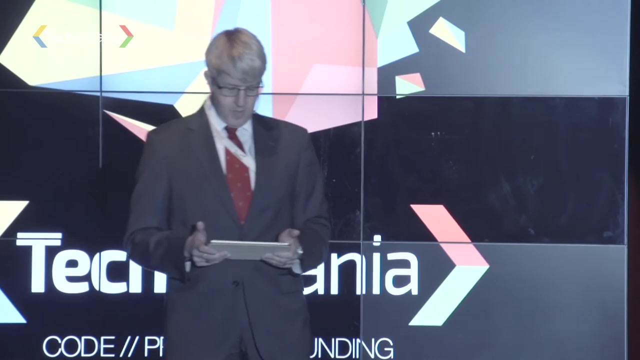 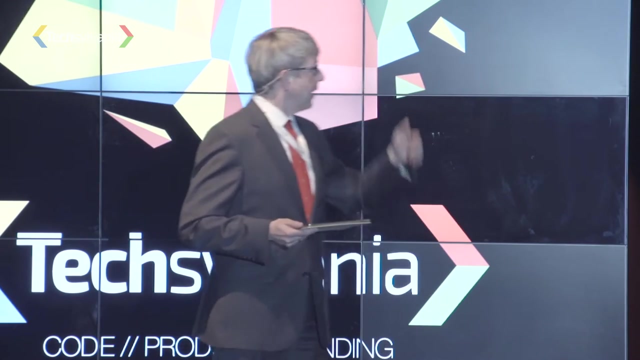 So, for example, technicians, When they look at some problem with some machinery, they might remember some similar piece of technology where they found the solution. They try to adapt the old solution. If you're looking at the doctor, looking at symptoms and identifying some disease by remembering past symptoms, past patients. 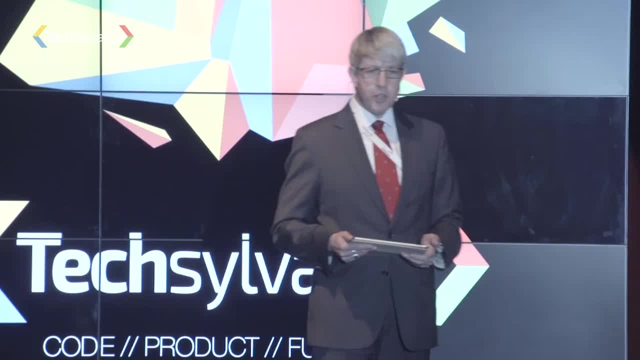 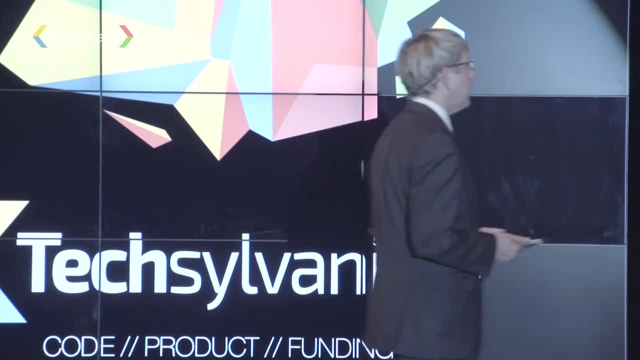 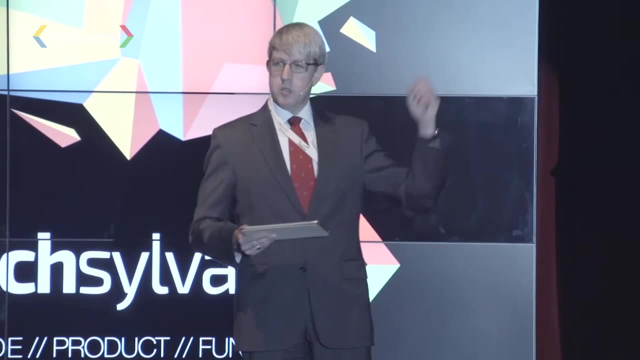 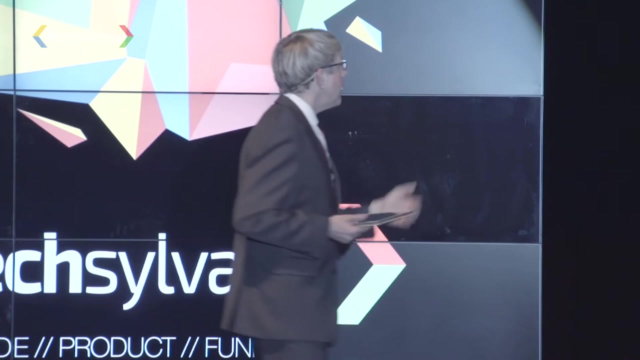 Or in law, especially in the American law, case-based law- Look at past cases that were helpful in winning a case and you apply them So we can use this kind of anecdotal experience and put them in kind of stories. A printer repairman remembers a similar failure of a printer in the past. 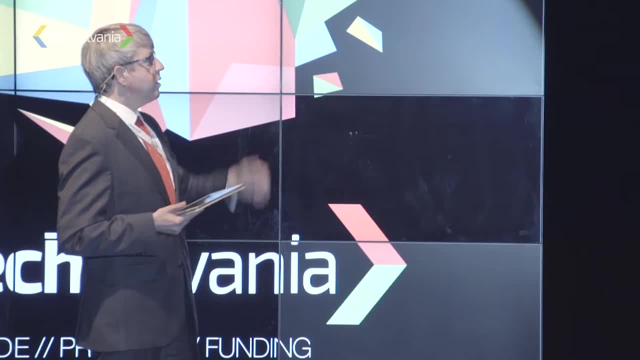 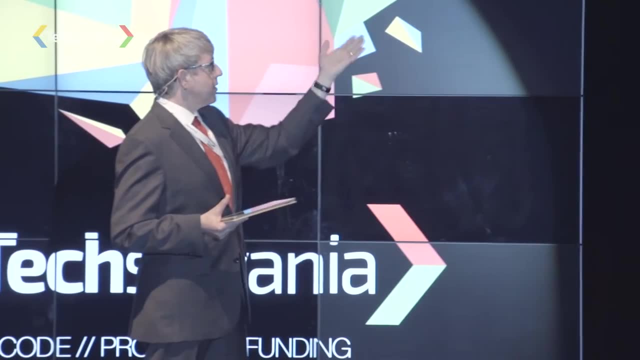 The problem was my printer has white streaks. I printed on paper. Cleaning the printer did not help. The solution was the ink cartridge was low in toner. The diagnosis was the ink cartridge was low in toner and the solution was to replace the ink cartridge. 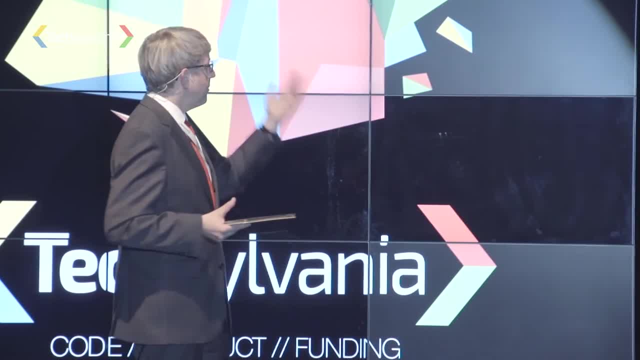 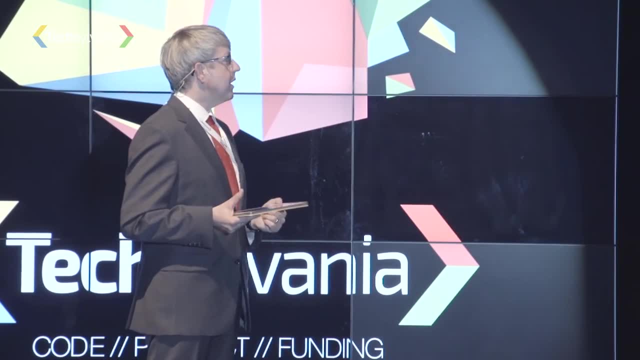 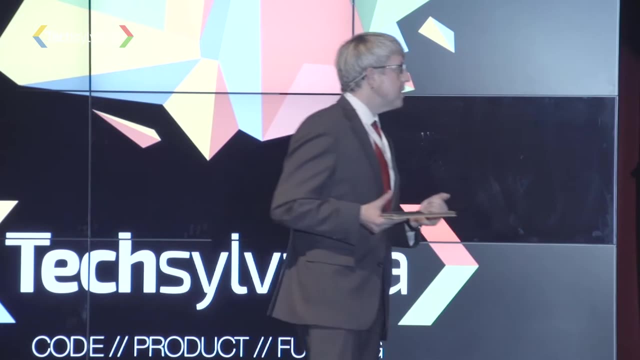 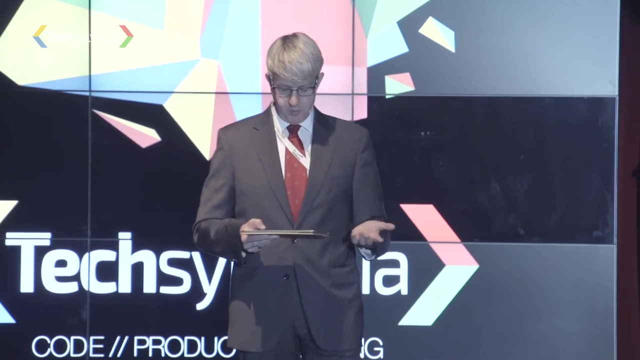 The doctor remembers the symptoms of a bacterial infection from another patient. The patient has fever, Blood tests show high count of white blood cells. Patient X tells about holidays in Central Africa And diagnoses: oh, it's probably some tropical infection And prescribes further blood tests and other things. 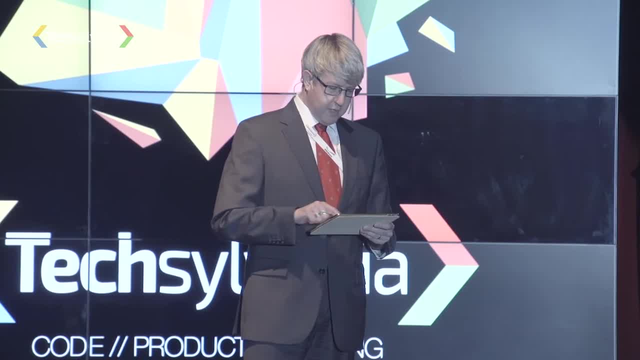 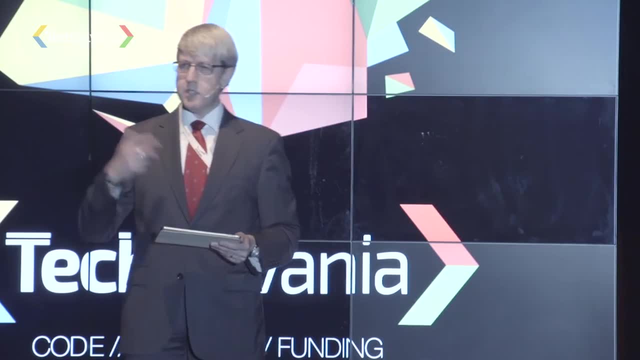 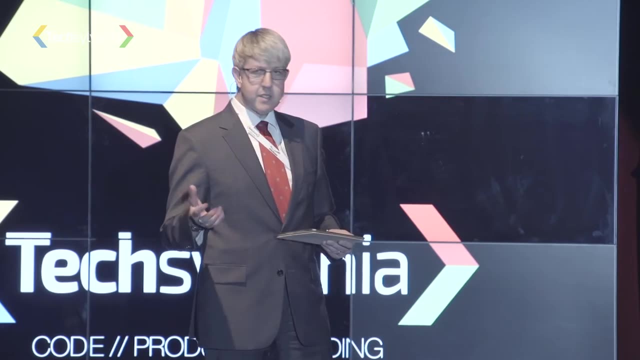 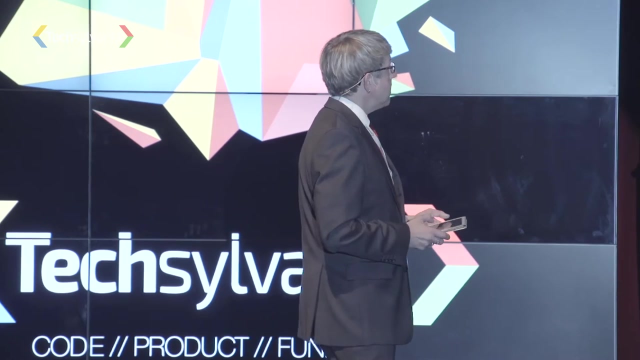 And the important part now is that these here, these individual elements, we can make more formal. We can put them in some formalism, Simple attribute value lists and object-oriented models And semantic nets, whatever you like, And we call these kind of elements cases. 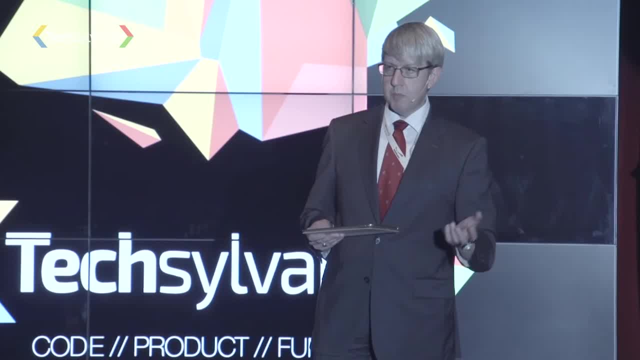 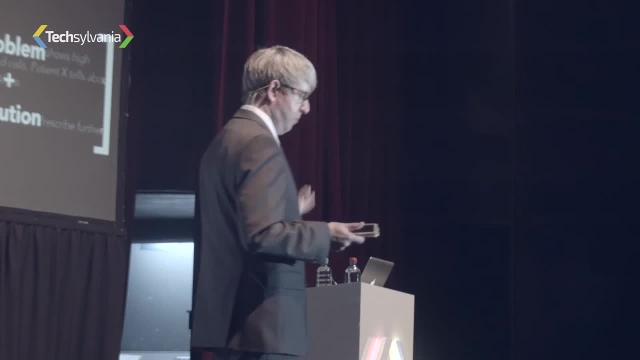 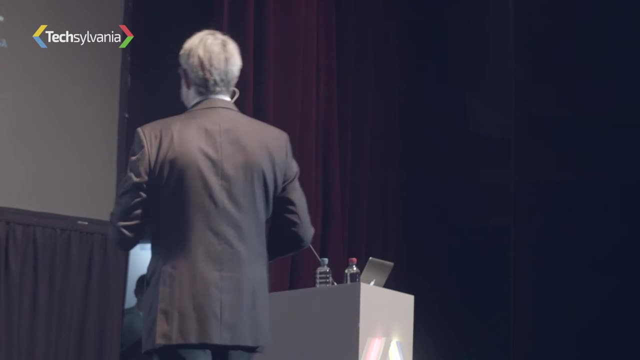 And the case in the traditional sense is a problem plus the solution, The same for our doctor's problems: Problem plus solution. So in that way, case-based reasoning is a cognitive approach. It's for modeling human problem-solving behavior, because that is how we typically solve problems. 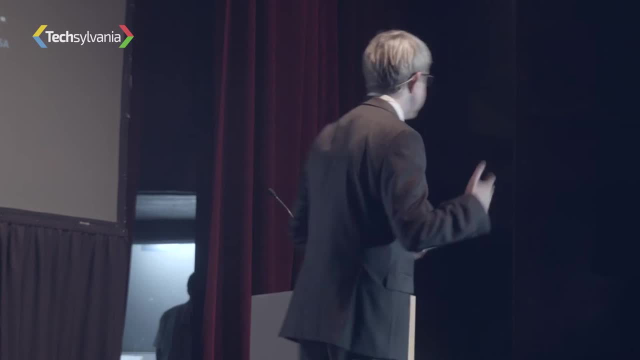 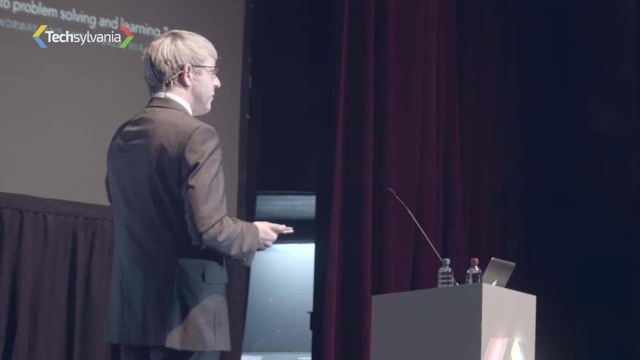 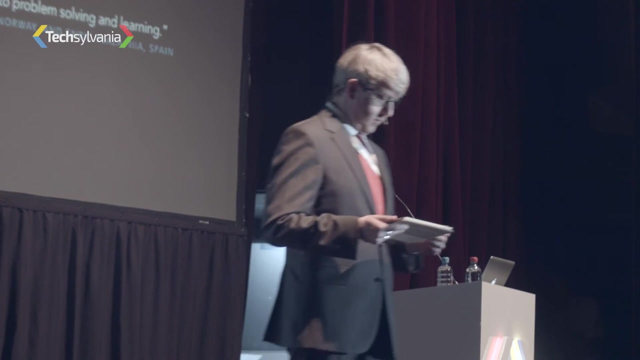 We don't go by textbooks, Remember similar problems and make something of it. So CBR is reasoning by remembering And we have developed that over many years into an engineering approach for developing and implementing intelligent systems. So it's an approach to problem-solving and learning. 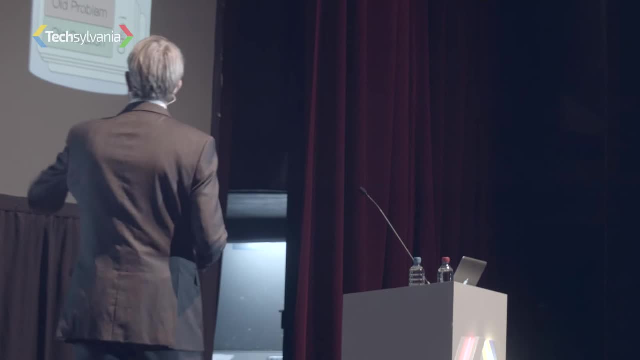 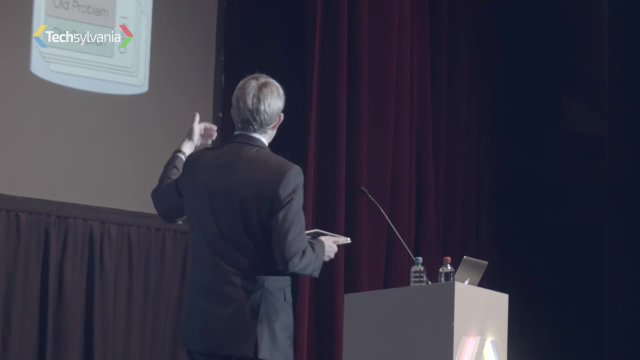 And the basic idea is really simple. You have a new problem and a so-called case base And you have lots of past cases. old problem, old solution pairs, But they prove to be useful. We try to find the best matching one. 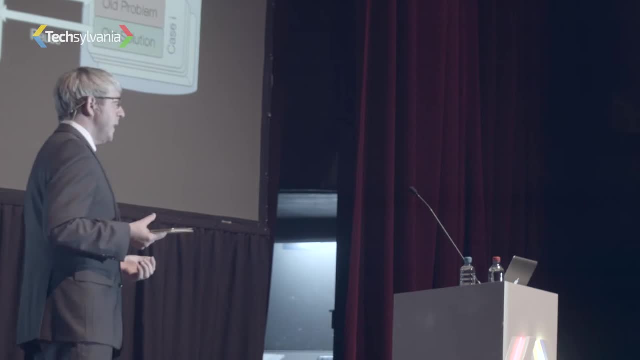 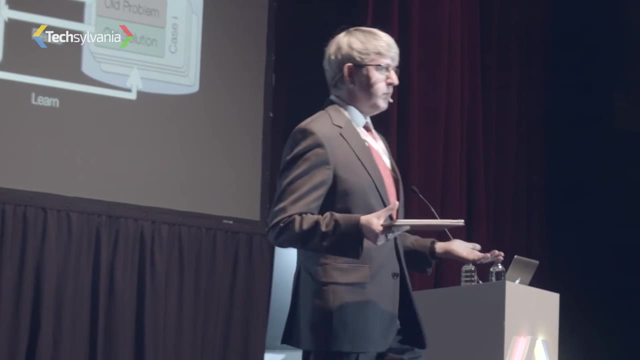 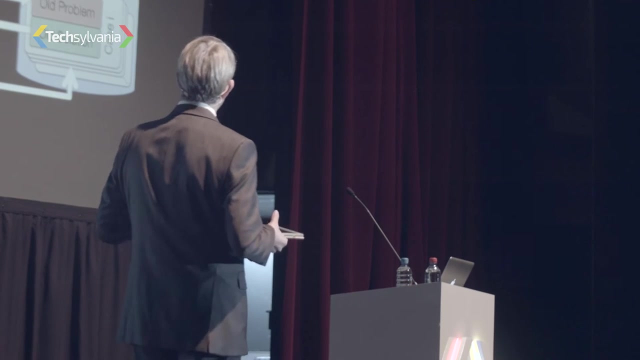 We use the old solution, Build from the new solution and the new problem, a new case, And you store it, You learn. That's the basic definition of any intelligent system: Intelligence: Ability to learn. So the key phrase here, the key aspect, is similarity. 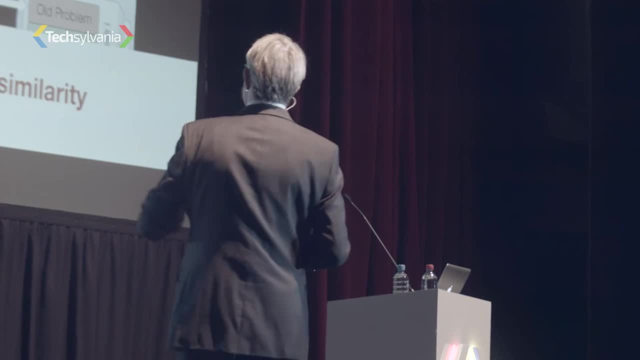 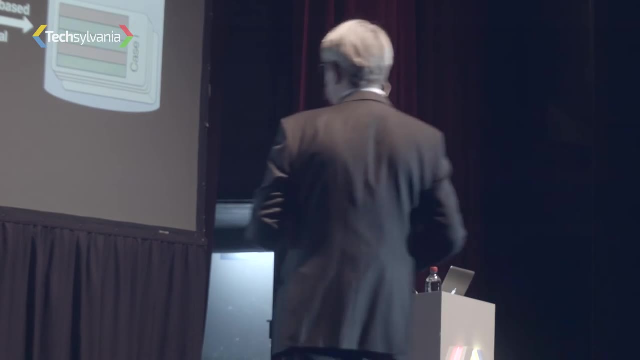 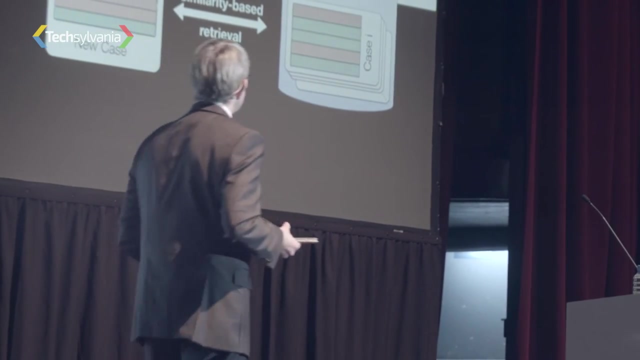 How do you express that? For recommender systems, we make the system a little bit simpler. You don't have- We don't have- the problem-solution pairs, But we have some specification, some requirements And via similarity-based retrieval, we look up the proper products and services. 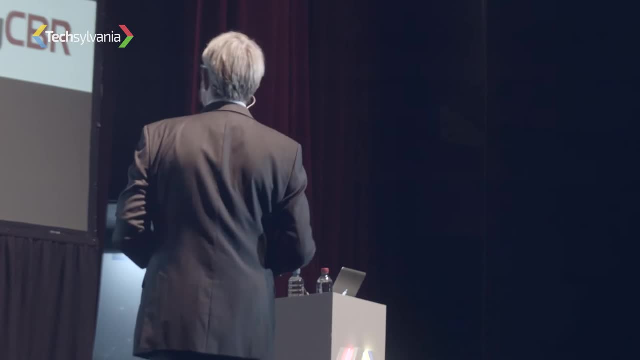 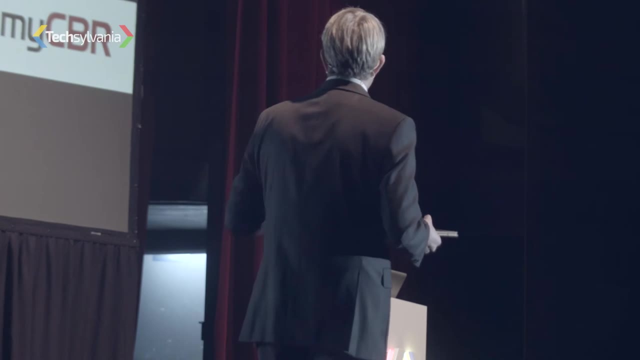 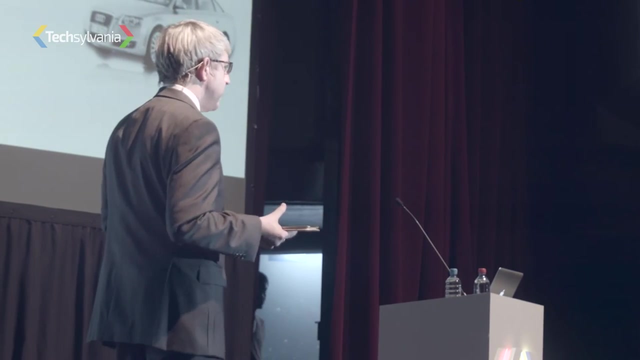 And to do that in a quicker way, you could use, for example, myCBR, An open-source software system that's available from my university and the German Research Center for Artificial Intelligence. Use it for recommender systems As an example. you want to recommend used cars? 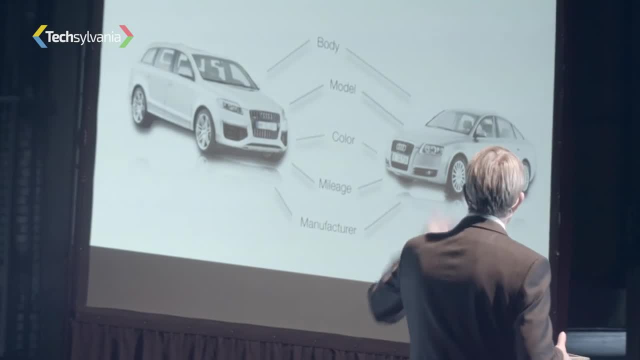 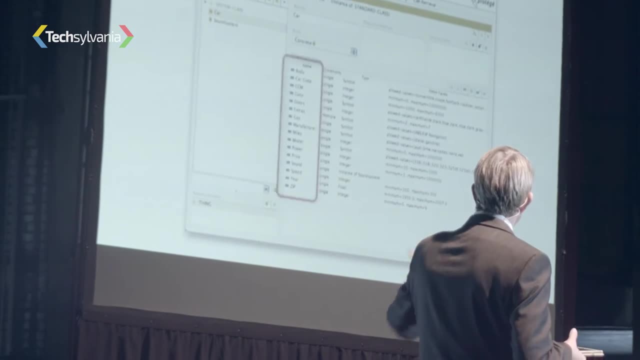 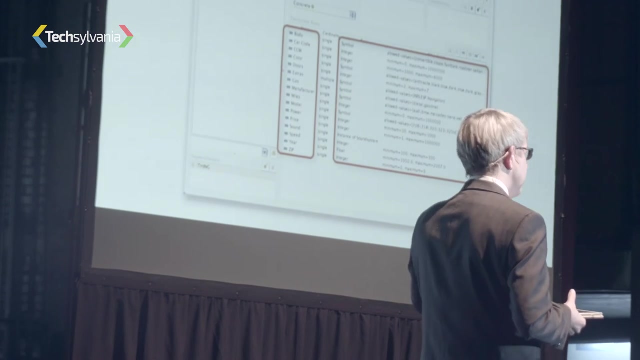 What do you do? You model your cars by body model, color, mileage manufacturer, for example. Put that in your system. You have your attributes. You have allowed values. That's an important bit for being able to describe similarity. You have to know what fits in into your attributes. 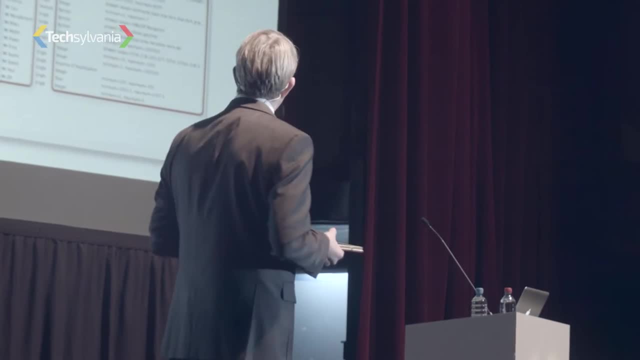 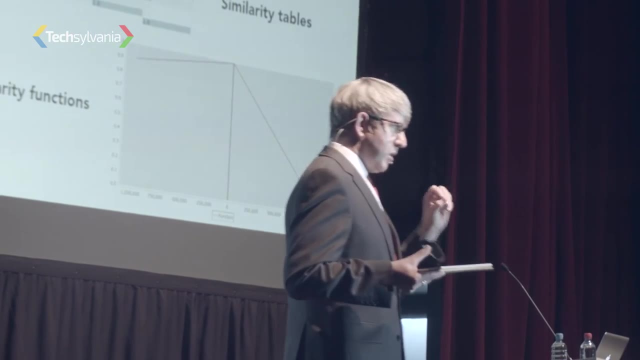 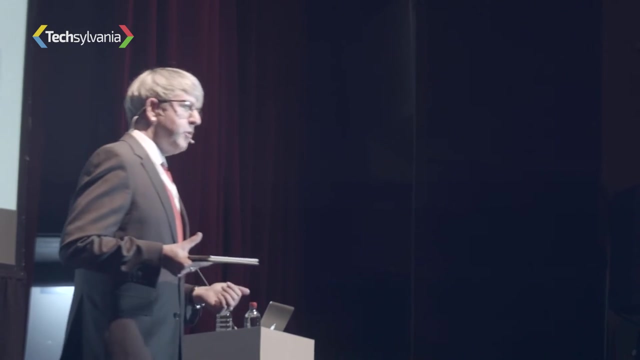 And you can even be object-oriented if you like And make more complex objects to compare The similarity knowledge needs to be told to the system. There are various ways of doing that, For example similarity tables. So if you know what kind of manufacturers you have, 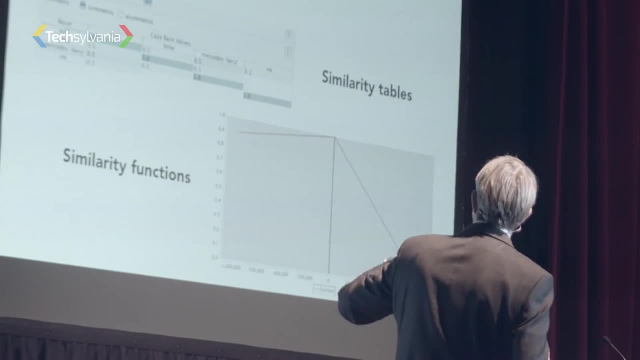 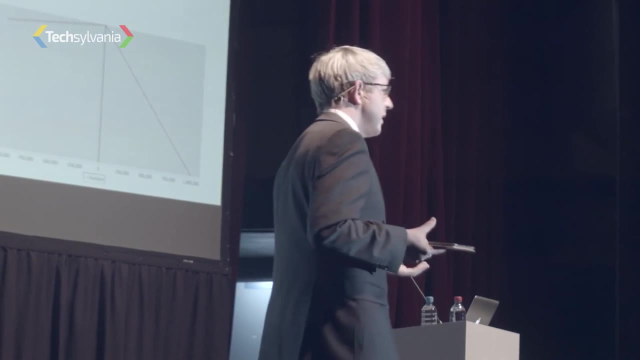 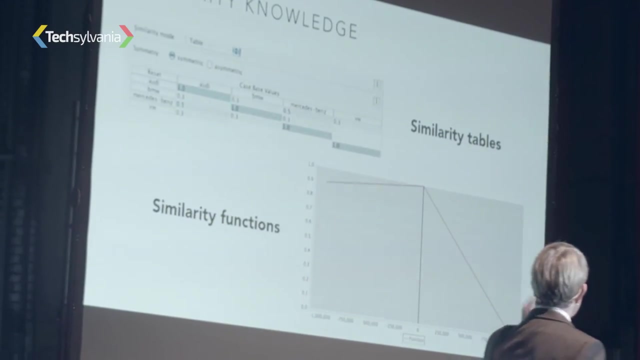 So Audi, BMW, Mercedes, Volkswagen, You could model how similar they are to each other. In the diagonal you would have 100% similarity And the other fields are somewhere in between. And for numerical values you can describe similarities with functions. 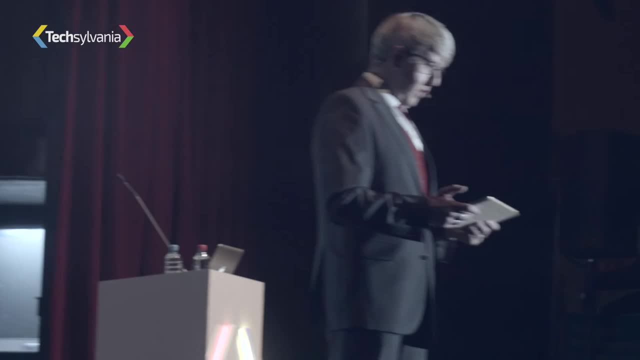 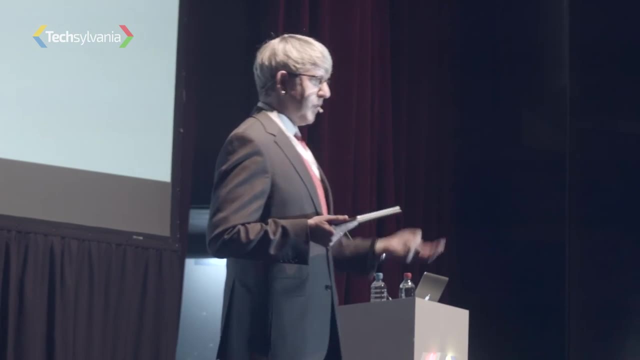 There are lots of ways of doing that, But I won't go into detail with that. Having modeled that into the system, you have the structure of the case, You have the cases in the case space and the similarity knowledge. You can then go for similarity-based retrieval. 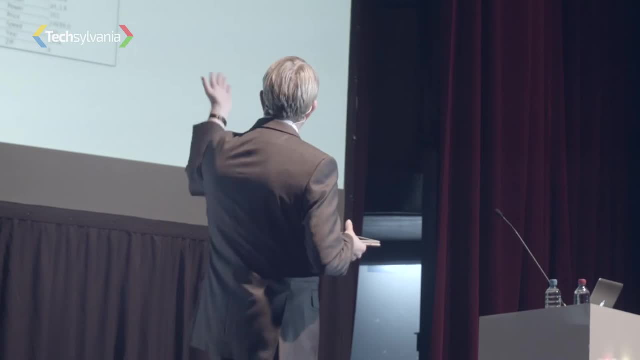 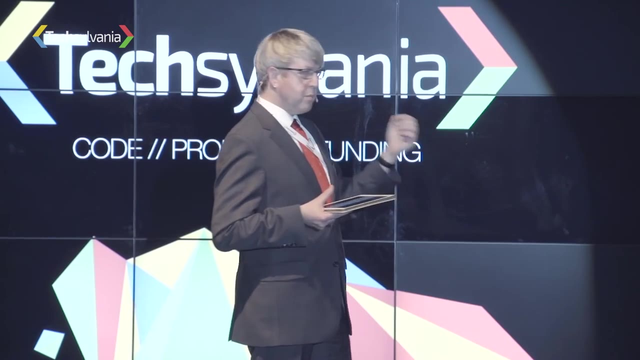 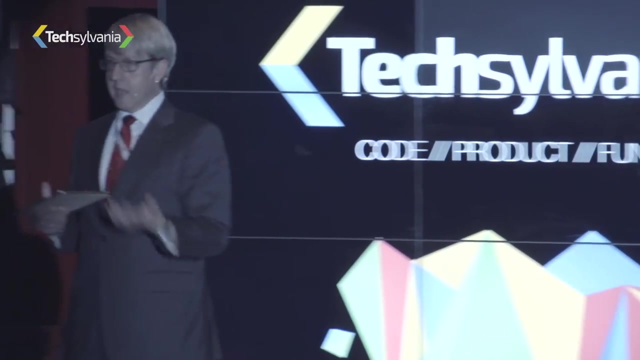 You describe your object that you're looking for Here. it's fully described query And you would get back from the system an ordered list of results. That's a big difference to SQL retrieval. In SQL retrieval you can only say how many examples you want to get back from the system. 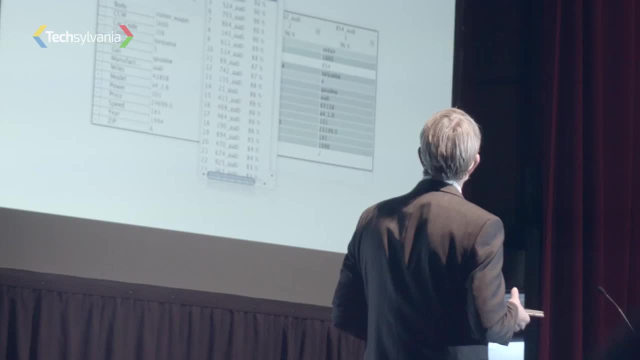 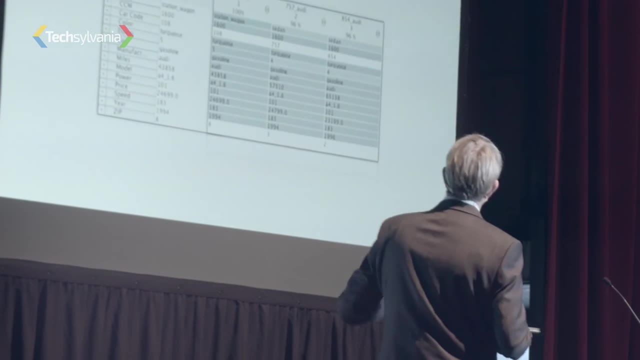 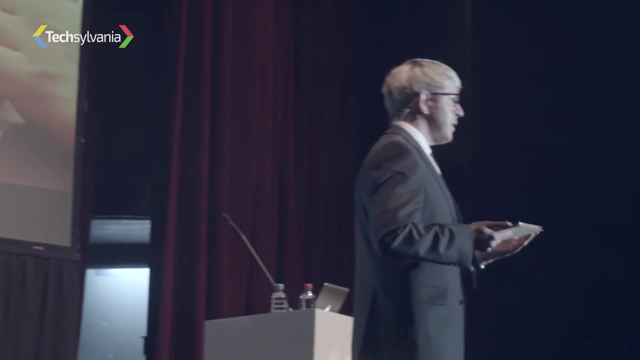 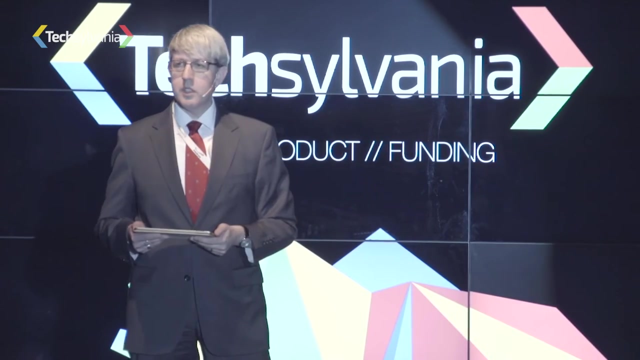 In case-based reasoning, you always get an ordered list, So ordered by their similarity to the system. That's a big difference. This was a quite simple example. Think about recommending experience from a recording studio. So that's one field that we teach at the University: Applied Sound Engineering. 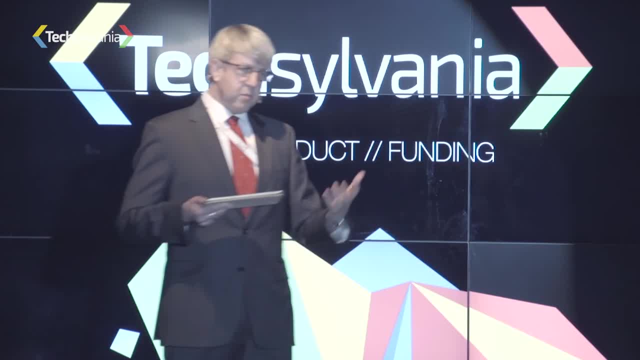 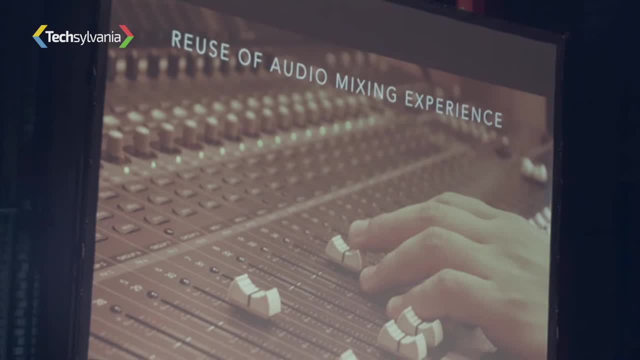 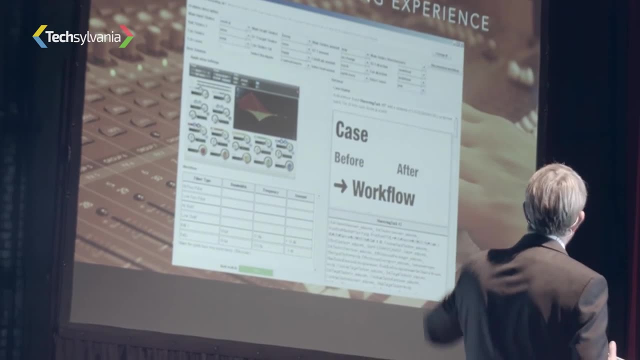 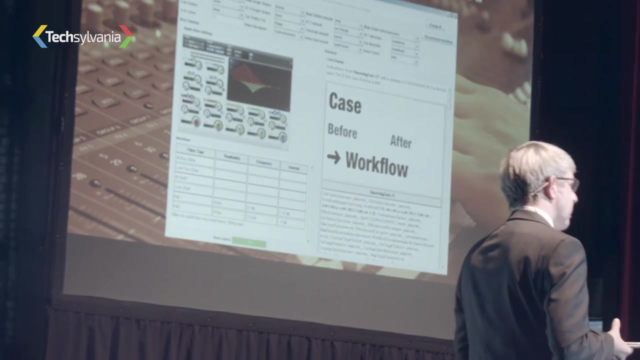 Students have to learn to identify certain kinds of sounds And how it sounds- tinny, hollow or rich- And to modify them. In this system, we build a recommender system that describes a lot of characteristics of a given sample And then recommend a workflow from something sounding tinny to something that's sounding more bassy, for example. 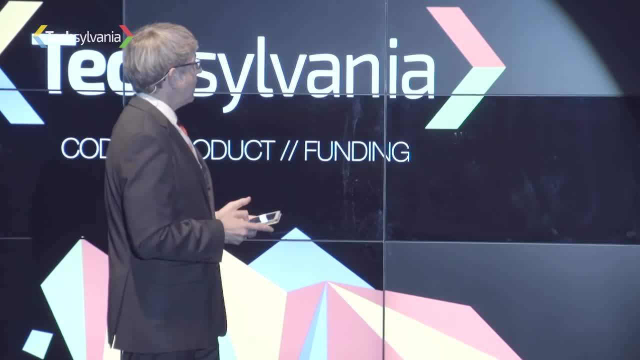 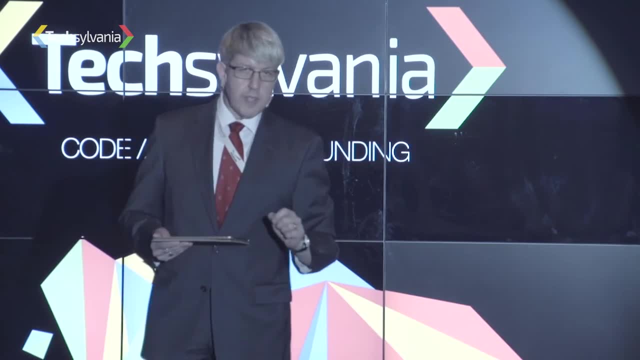 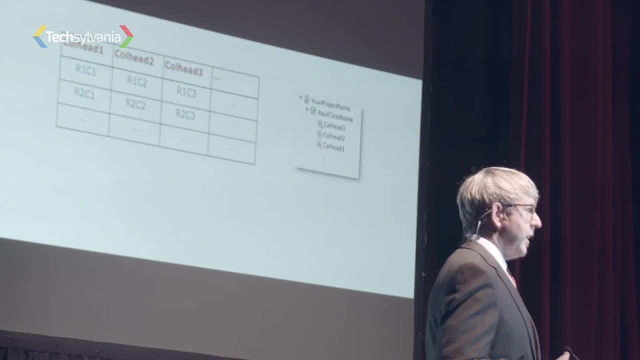 And that is suggested as configuration for the recording system. And to make it more techy so that you can use myCBR, if you want to, and try it out, we have built also a comma-separate value list importer which allows you to build quickly your initial model. 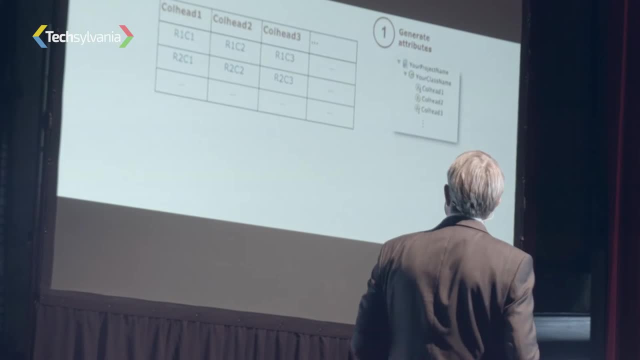 Let's assume you have this CSV list with column headers. You can generate attributes easily from the column headers because you just take the names. Then you look into the columns for the data types and guess from it. It's a symbol, is it a boolean, float, integer and so on. 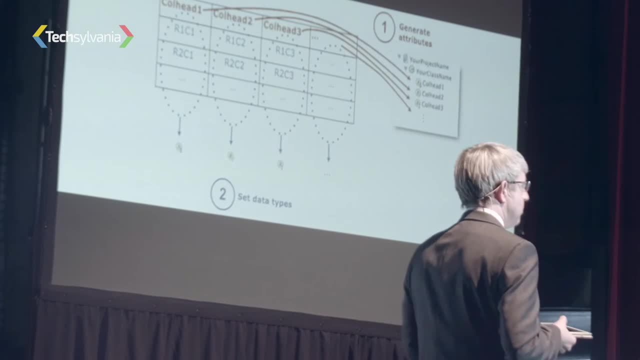 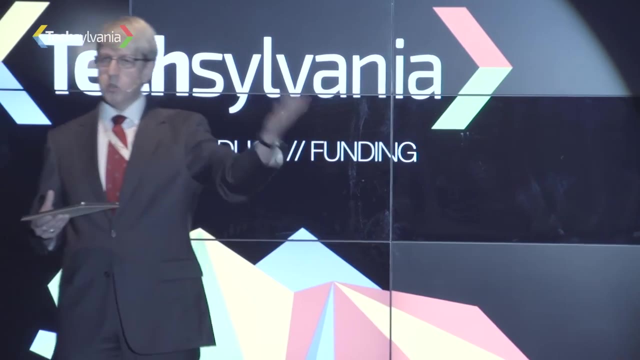 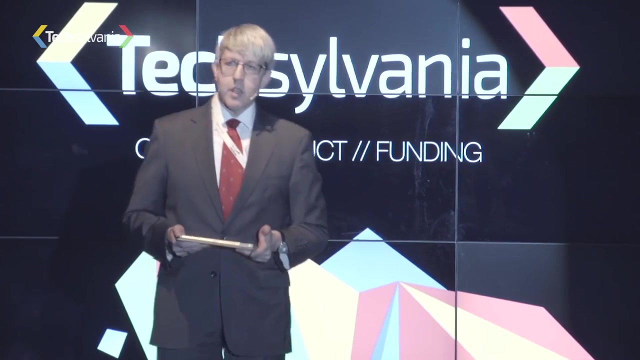 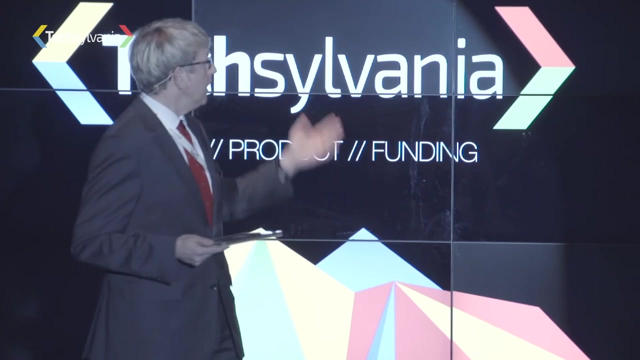 And generate from that the initial model. At last you generate the instances and you have a case space. You can then go right away to your similarity measure editors and try out if that works how you want. If you want to know more, go to that URL, download your copy, try it out, play with it and give us feedback. 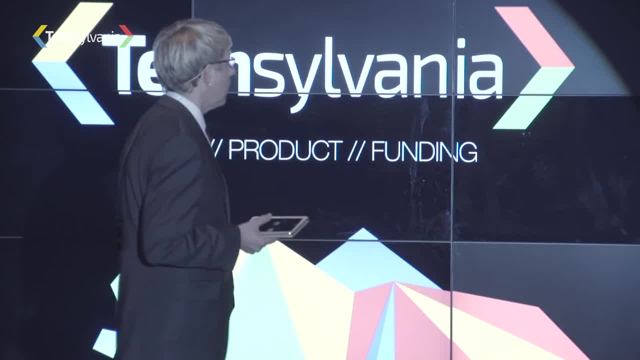 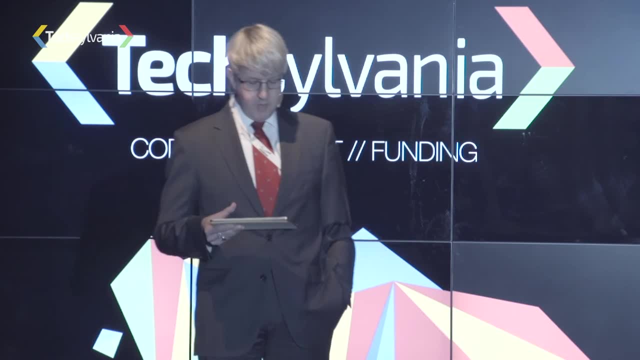 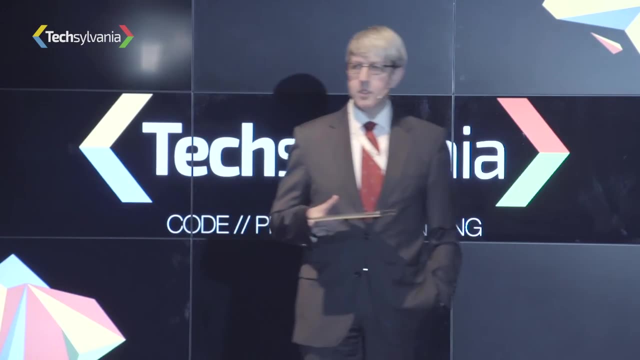 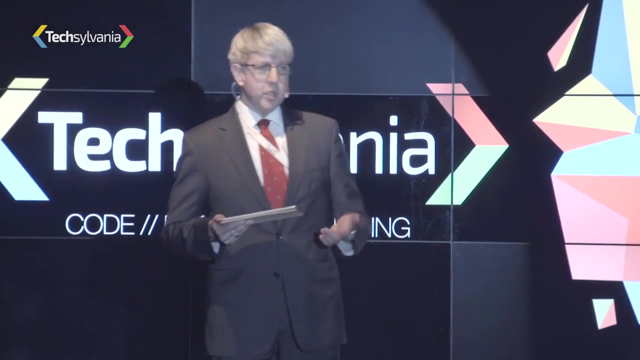 So what are my take-home message of this brief talk? Case-based reasoning is the method of choice whenever you need to compare products and services That might be products like on Amazon. So it's content-based comparison compared to collaborative retrieval, which is how Amazon has implemented most of their recommendation system. 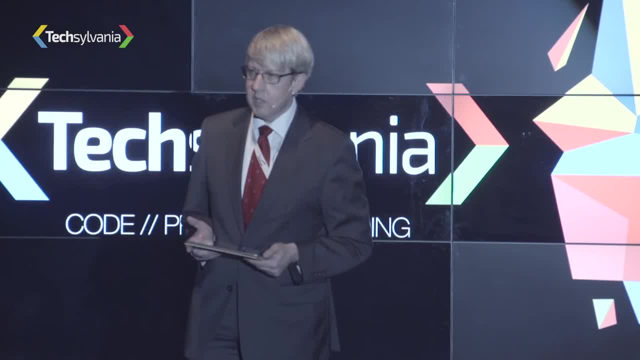 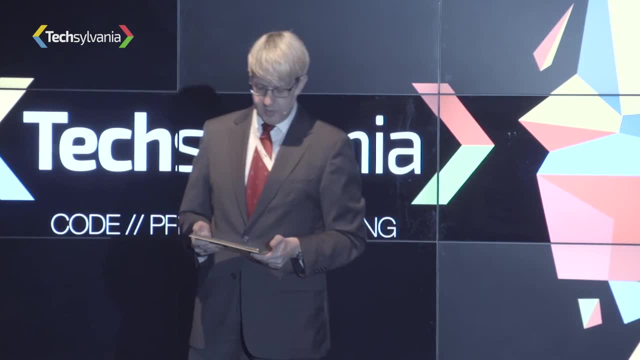 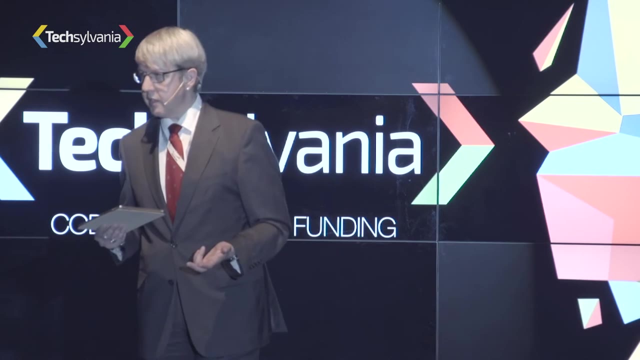 They are just looking in the basket, what they have, what other customers have bought, But here it's looking at the characteristics of a product. But think wider, Think about other things on the web, Think about web services And think about the Internet of Things. 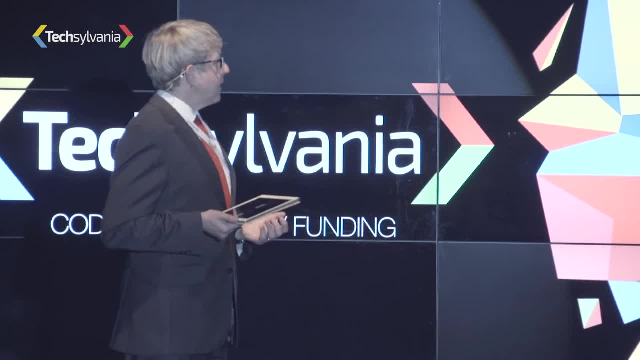 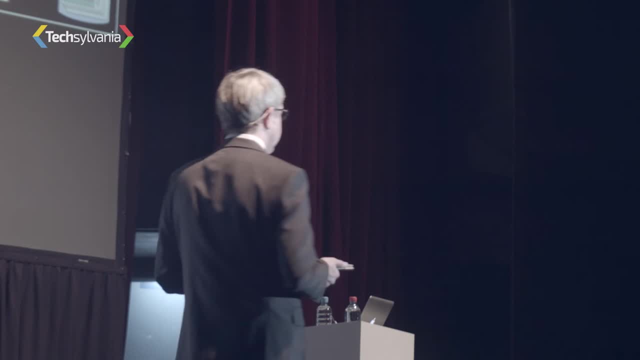 If you are in a system or in a web that is unreliable to some degree, you need to have other services that you use if one is not available. If you have the characteristics of the service that you need, you could use, for example, myCBR. 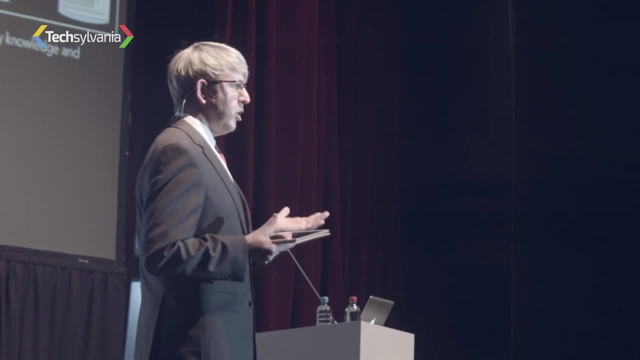 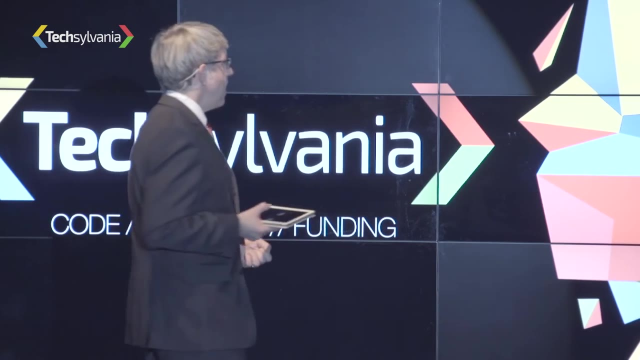 for doing exactly that: Build your knowledge model, Build your similarity measures for it And have a lightweight system to give you other products and services or access to devices. If you have modeled with myCBR Workbench, so that's our graphical user interface for it. 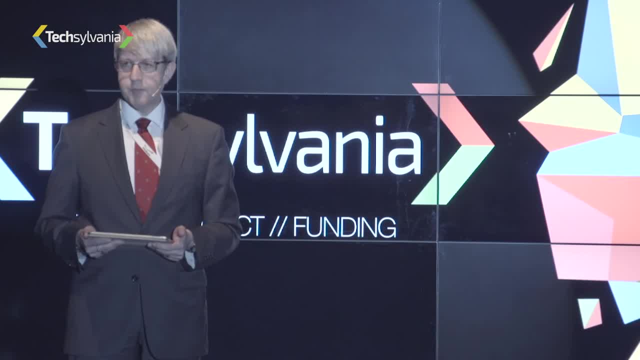 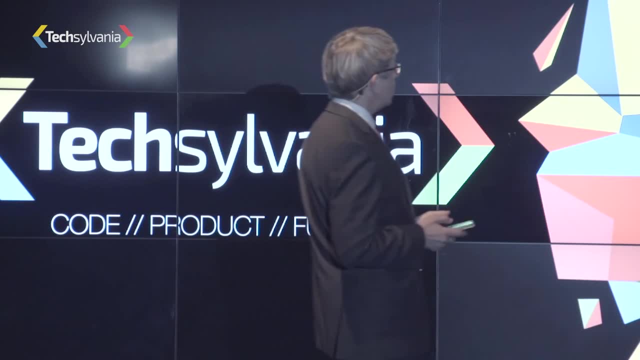 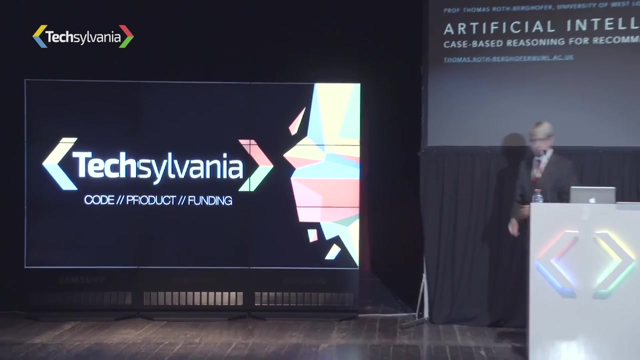 you can then use just the SDK to implement it. It works also on Android phones. We had some master theses that worked it out. Thank you for your attention. Thank you very much, Thomas. So I took a lot about learned from that. 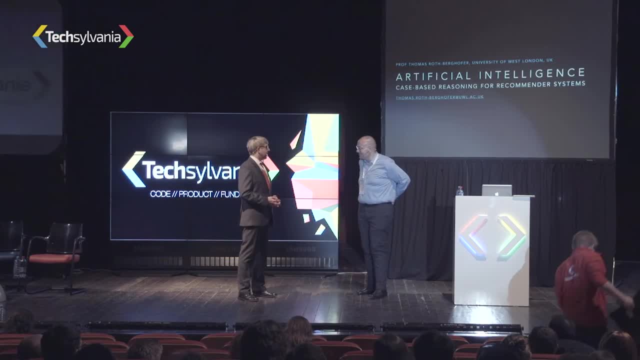 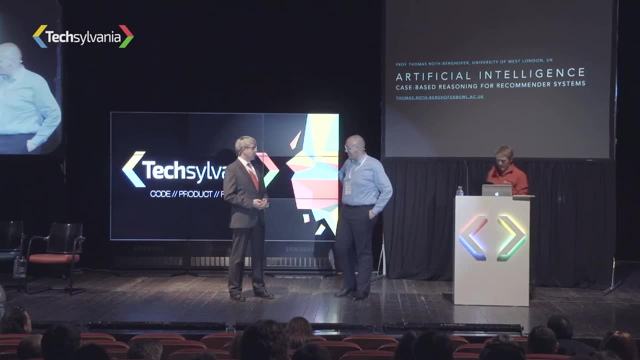 So, with the great tools that you built, I have the feeling that even I could start building something in artificial intelligence, Absolutely So. yeah, My programming days are long over, but it sounds like I should like jump a wave and go directly to artificial intelligence. 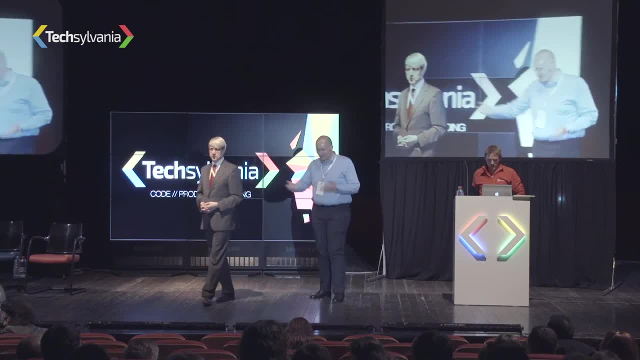 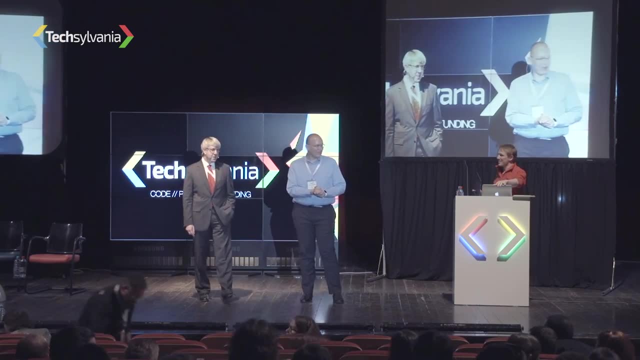 So that's fantastic. So since you managed, like in good German fashion, to finish like in time, we'll have time for asking a couple of questions from the audience while our next speaker is setting up. So there's a question over there. 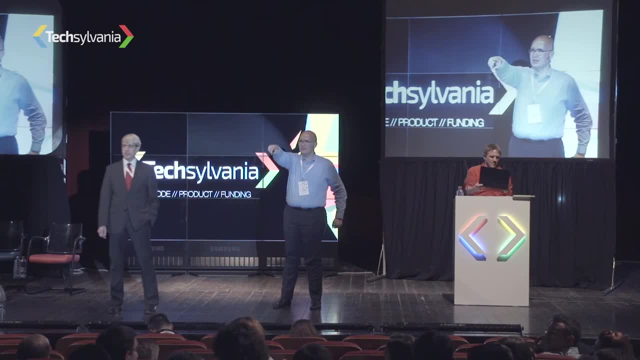 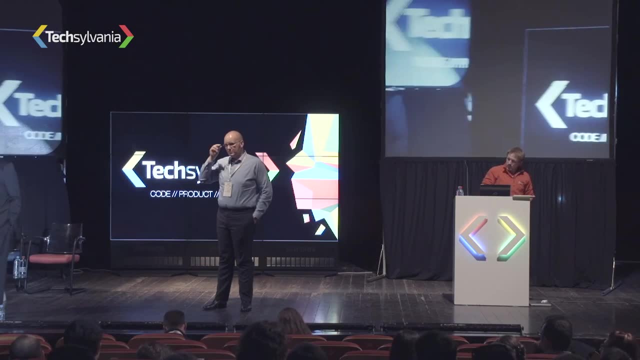 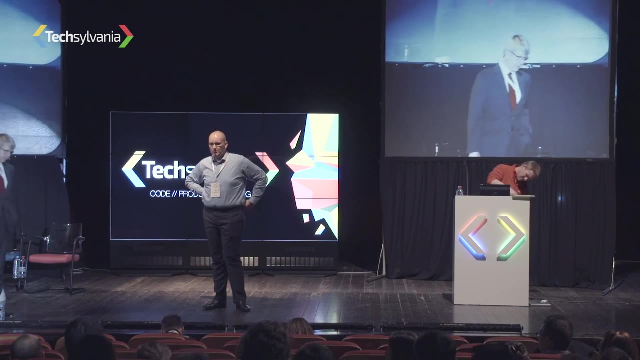 So can we have somebody with a microphone going there? Yeah, somebody with a microphone is coming. Okay, So my name is from Accenture. I have a question related to this learning process. So, from what I understood, the learning can be automatically done by the artificial intelligence. 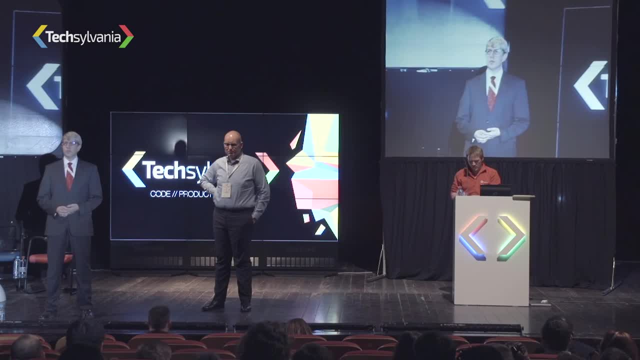 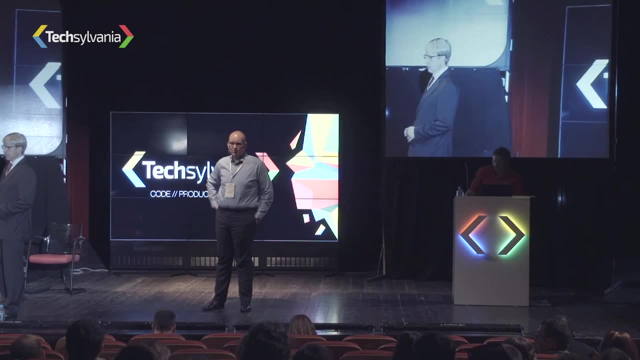 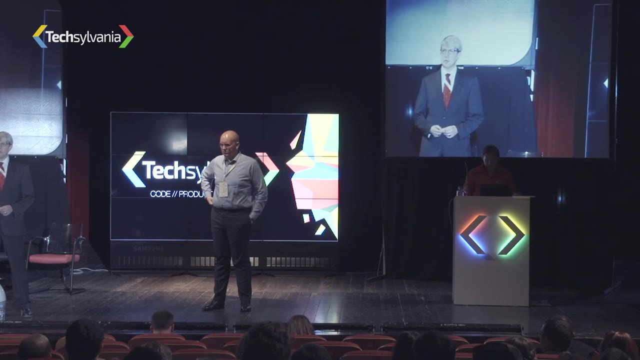 so with the new case that has been matched to an existing case in the database, What about if you have a new case and that case contradicts with existing cases? Is the system able to unlearn some existing cases or correct them? So that's one of the things. 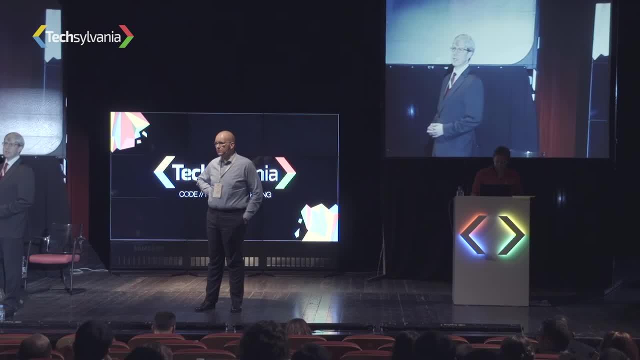 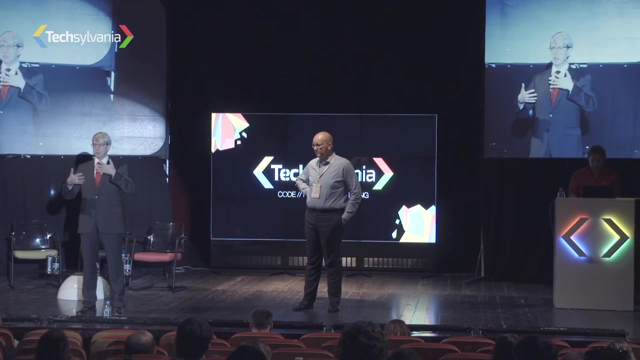 You don't have this concept of contradiction in that way, Because if something is contradicting in your similarity model and that was too short to show you how the similarity is calculated, it would have a very low similarity measure. So from the point of view of retrieving this contradicting case, 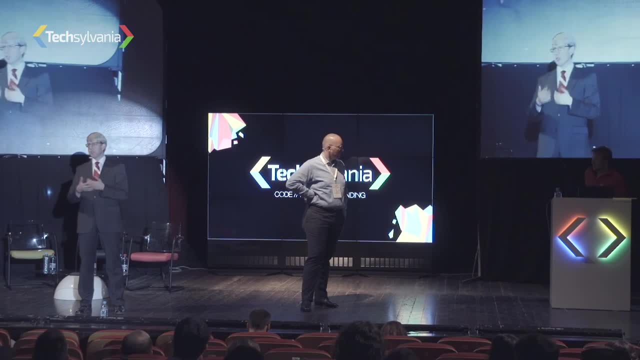 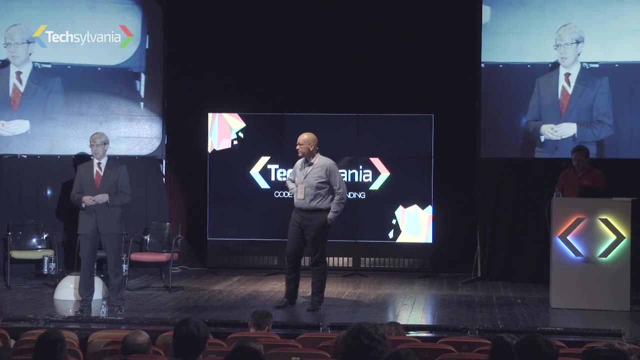 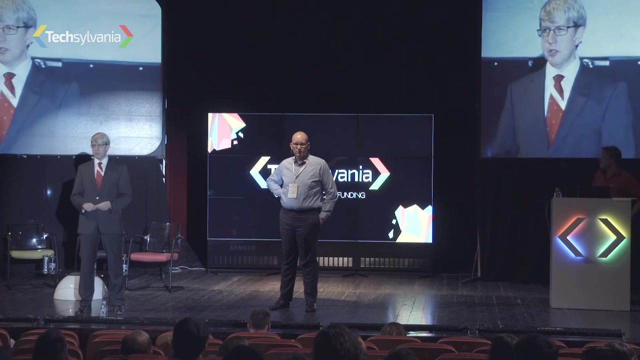 it doesn't affect the retrieval in that way, But it's exactly a point where knowledge maintenance is important, so that you have scripts, queries that run over the case base and find out extreme values, Or, in that case, when you solve the problem.